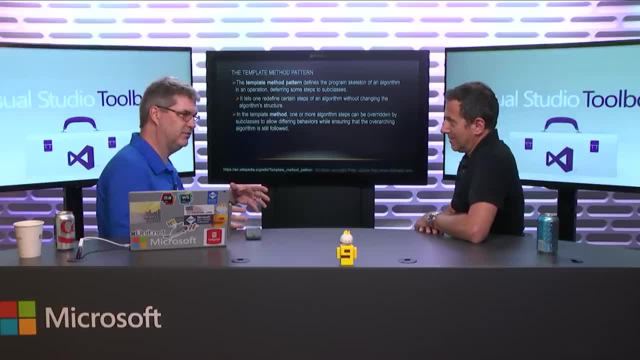 cut the pizza box, the pizza. Well, we got to box it, Box it Right. See, that's where we have a template, Assume. well, maybe, or plate it Or plate it Right. Well, let's say it's going out for delivery. 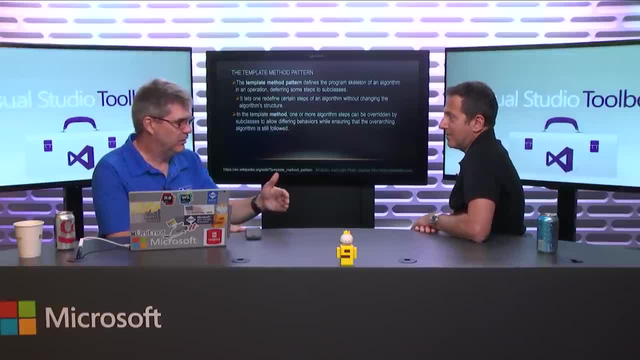 Yeah, So you don't want to get that order messed up. No, Right, You don't want to put it in the box and put it in the oven. That would be bad, Right, Right. So we want this, But that can't possibly be the pattern. 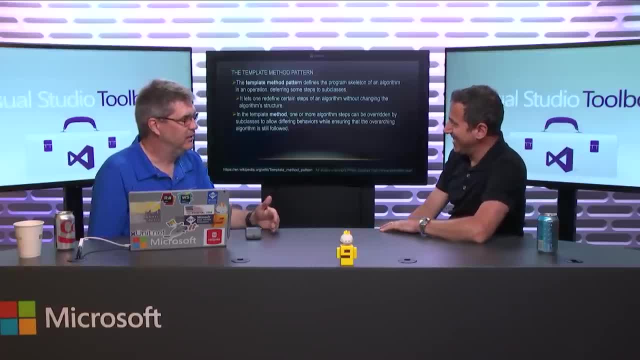 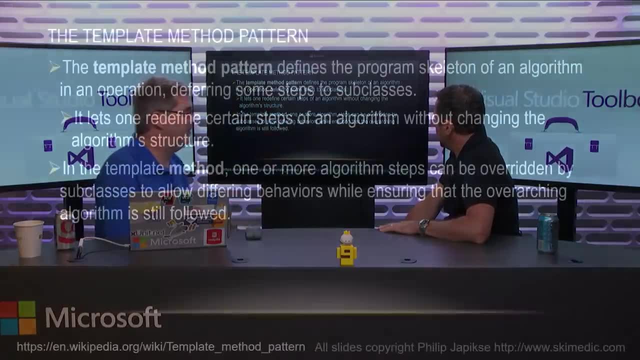 No, that's not the pattern. Do things in the right order? No, But that's part of it, right, So we've got this template to do things. Yeah, Right, So defines the program skeleton of an algorithm. So the algorithm is. 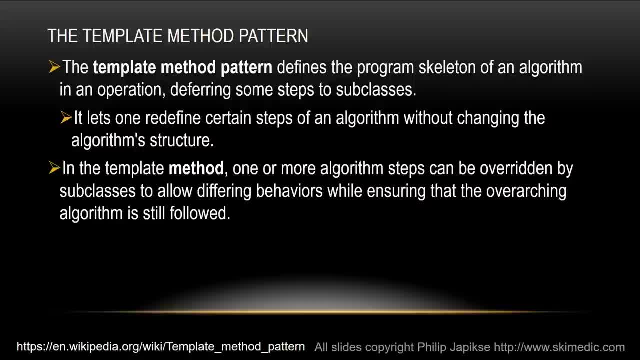 how are we going to make this pizza? But it's the deferring some steps to subclasses, That's the pattern, That makes it part of the pattern. That's the pattern, Because if it's just, oh, what are the five steps you need to do to make a pizza? 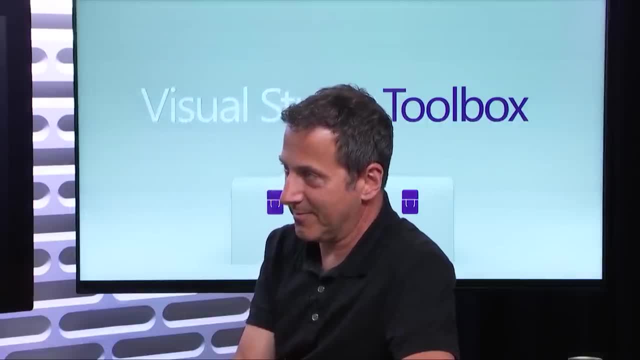 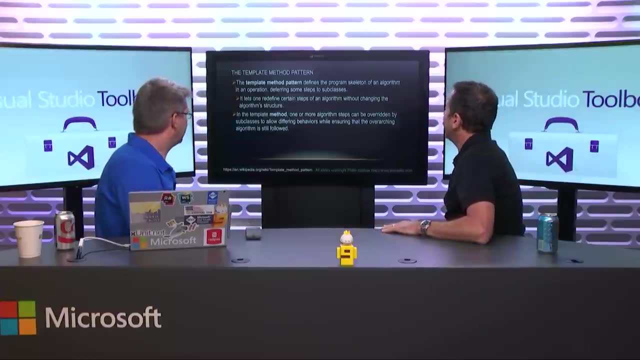 Get them in the right order. That's not the pattern. No, Because you could do that with the command pattern, Right, Right, You can do that by writing the right code for crying out loud: Well, yeah, Okay, So you can redefine certain steps of. 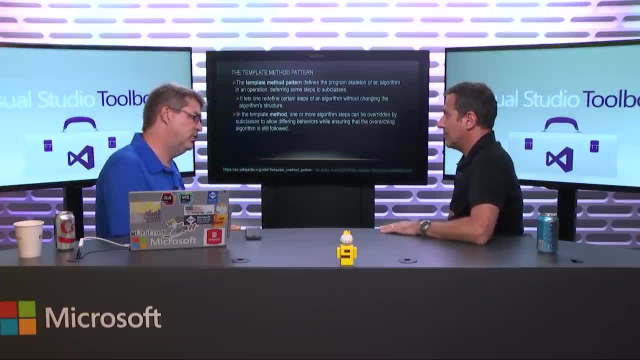 an algorithm without changing the algorithm structure, Right? So let's say, if cooking the pizza, you're only going to half bake it, or you're going to twice bake it, or things like that, right? So a derived class can change how that particular step works. 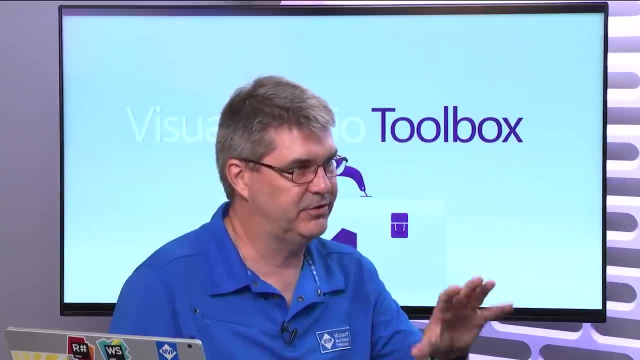 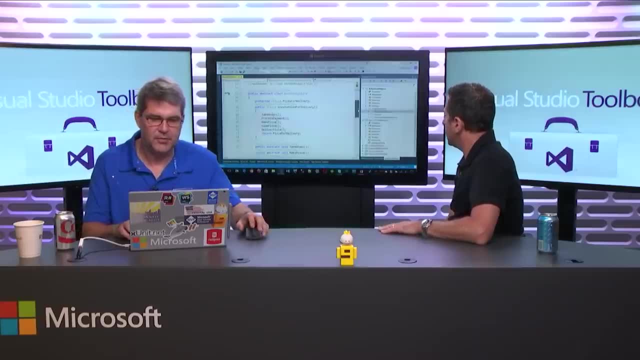 Okay, But I haven't rewritten the algorithm. The algorithm itself is still the same. Cool Right, Right, All right. So let's look at the code, And this is one of the rare ones where I don't have unit tests around it. 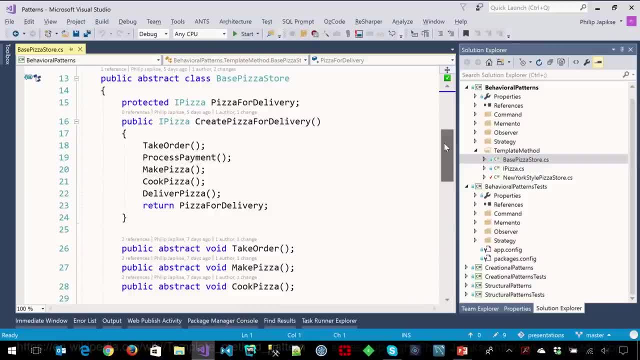 but it's a pretty self-explanatory pattern. But I think there's a lot of- It's pizza. It's going to pass. Yeah, There's a lot of it. Pizza is good, right? It's how you get all the developers in one room, right? 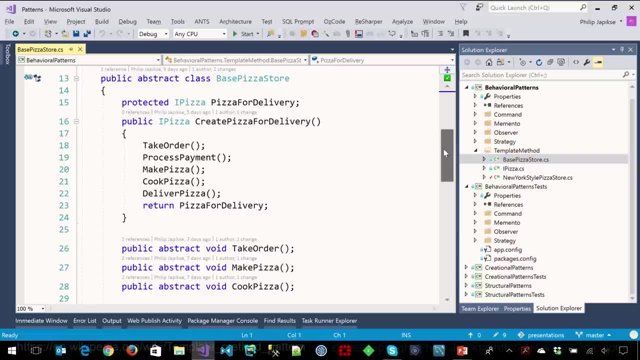 You bring in free pies. So here's my abstract base pizza store. Okay, And I have to think, and you know what? We haven't been mentioning resources in the other episodes, but one of the things that we're going to put in is a link to 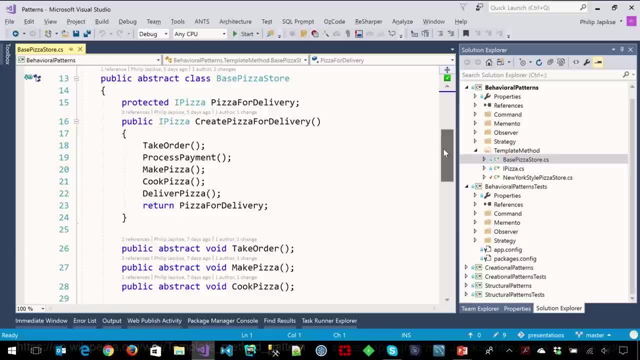 the Head First Design Patterns book and we'll put that in all the show notes. That's an awesome book, So I want to thank them for inspiring the whole pizza theme that we'll see in several other patterns as well. So here are pizza steps. 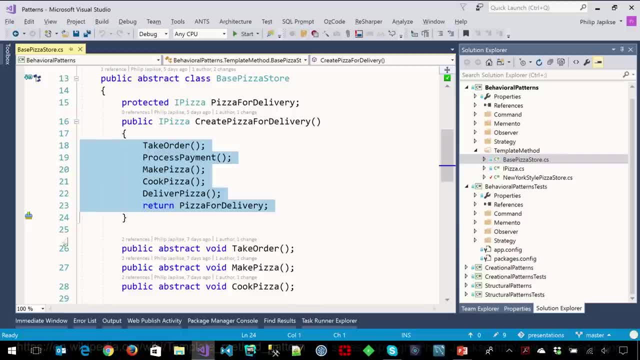 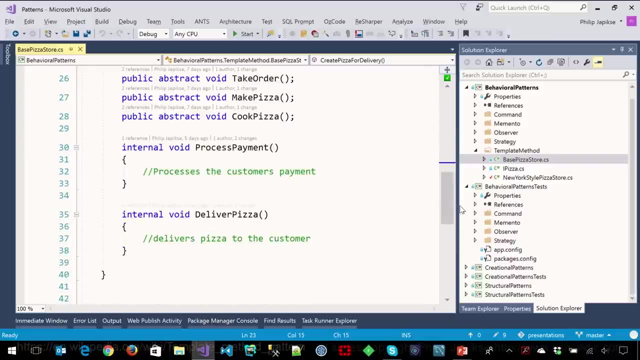 Take the order, process the payment, make the pizza, cook the pizza, deliver the pizza, and then we're returning this out of the- Mm-hmm, Out of the method. Didn't really need to do that, Okay, But we are, and we've got some things that aren't going to change. 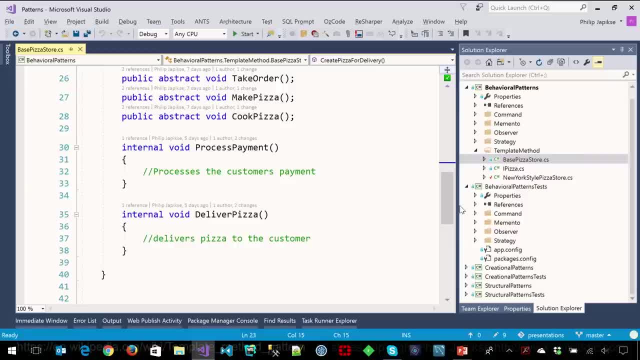 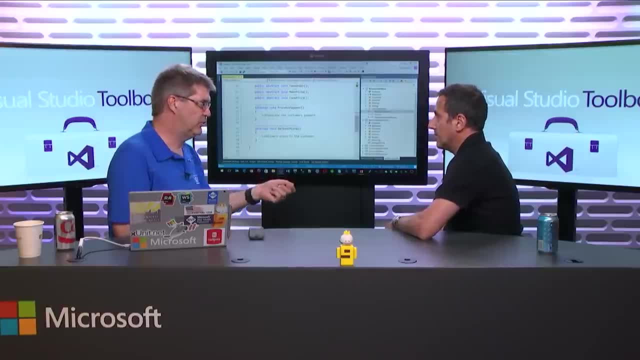 regardless of the type of pizza? Right, okay, Processing the payment and delivering it happens the same. Yes, Regardless of the type of pizza, I'm going to charge a credit card, I'm taking cash. However that works. calculate the price. 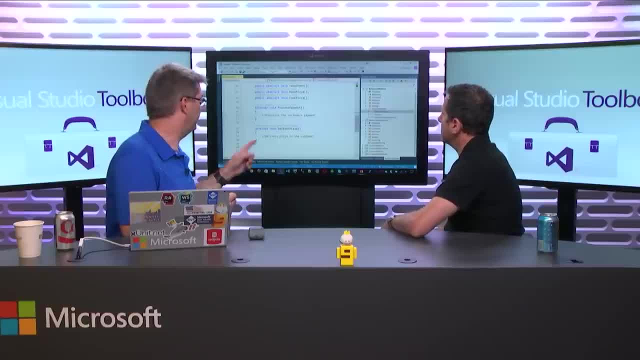 Calculate the price might be something that varies, but it's not actually processing the payment, And delivering the pizza is the same across all pizzas as well. It's entirely possible that, depending on the pizza you make, You could deliver it differently, but- It is possible, and then you would have to extend this to override that. 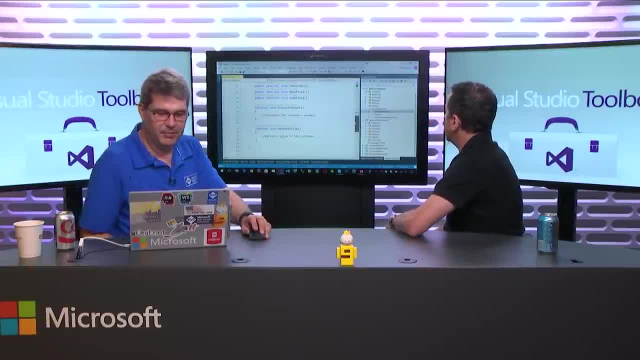 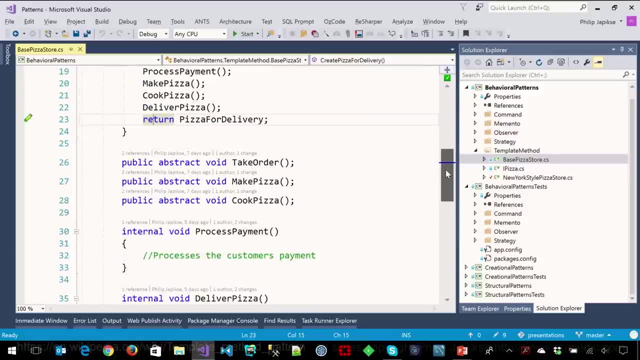 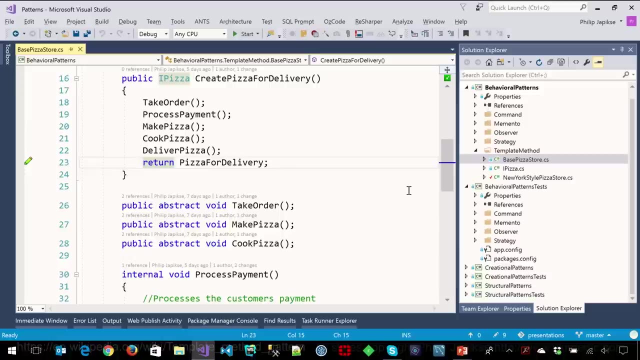 Yep, Right, Okay, So we've got these base implementations for processing. So it's the fact that take order, make pizza, cook pizza. that's always going to happen, but how it happens can be different- Yeah, different, and therefore you put it in an abstract class. 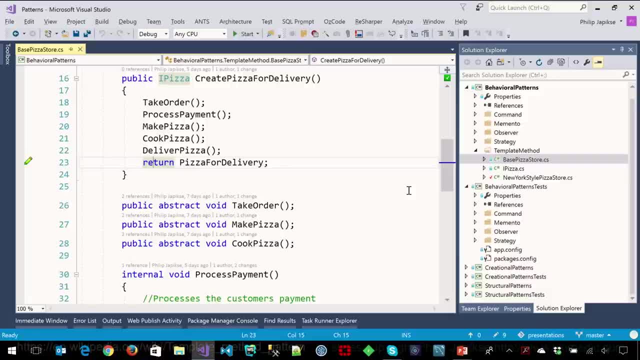 that's what makes this the template method pattern. Yeah, and to be clear, it doesn't have to be abstract. I could have made those virtual and have a standard implementation which, for example, we could have done with the deliver pizza. 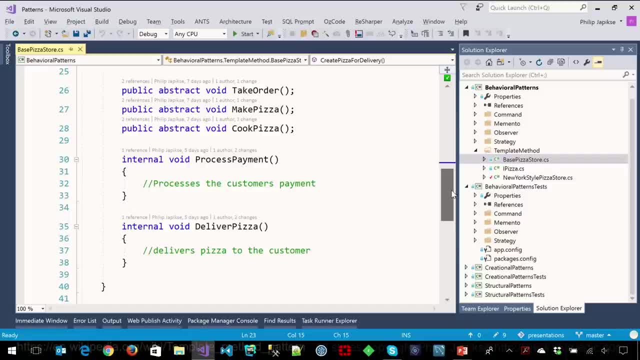 So if it's a hot pizza, it's always delivered the same way. But let's say you're going to deliver a half-baked pizza, the one that you finish cooking at home. Maybe that has a different delivery style. Maybe it has to be refrigerated, who knows right? 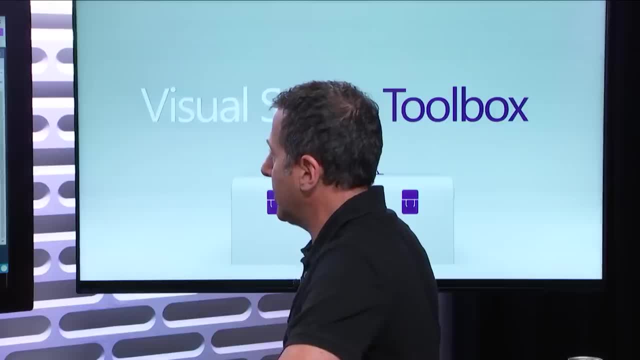 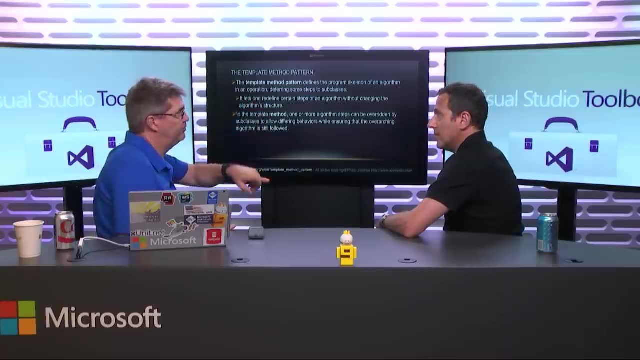 But the fact that the implementations of these live somewhere else and are brought in at runtime. that's what makes this the template method. Going back. well, they're actually brought in at design time, not run time, cuz we've got these classes built. 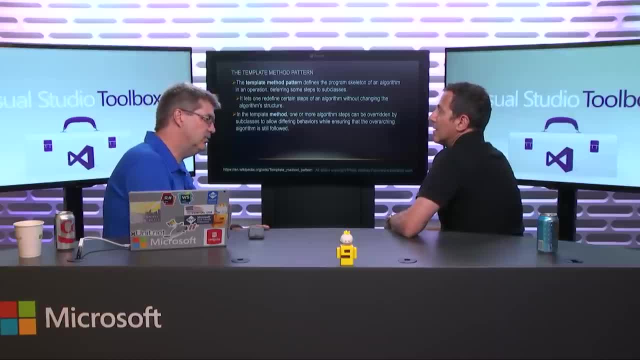 We're not changing the implementation at runtime. Okay, We're defining the implementation at design time. At runtime, we could pick a different-. Yeah, yeah, yeah, Yeah, We could pick a different style of pizza store, But that's not the strategy pattern. 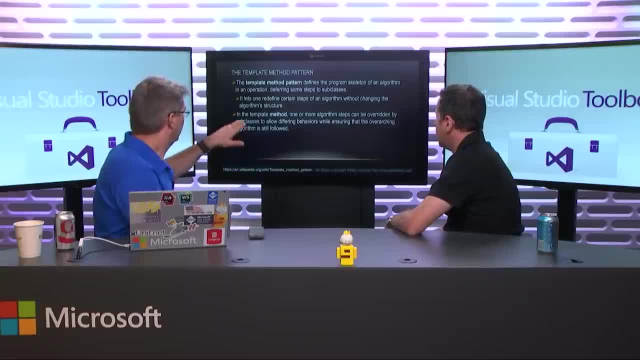 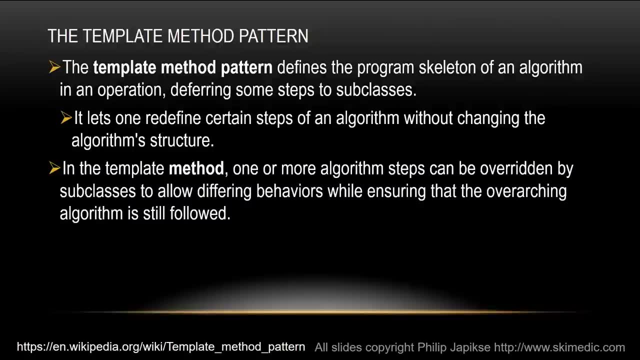 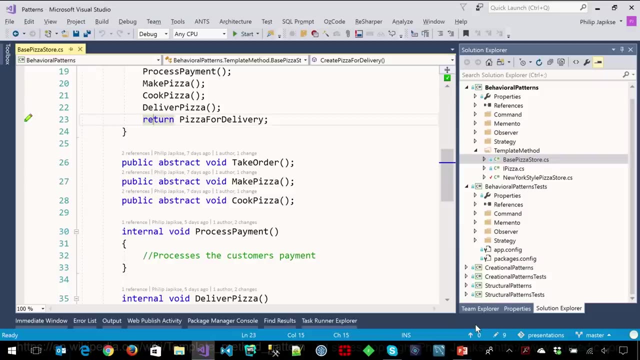 We're just picking a different implementation. Okay, Right. So again we've got the program skeleton defined and we're deferring some steps to subclasses Mm-hm. So we've deferred the make pizza, cook pizza and take order to a subclass. 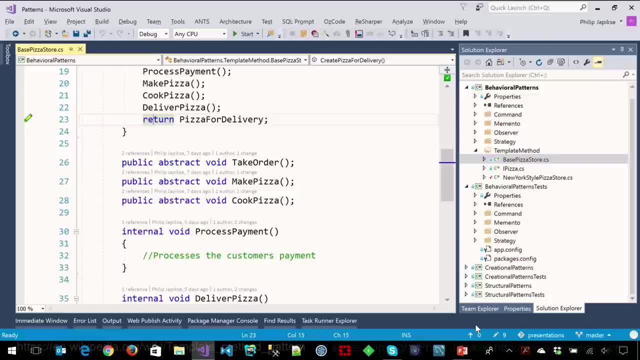 Okay, Now the reason to take order. I love my Chicago style pizza, Mm-hm. My wife loves the New York style pizza, but you take the order differently, right, Cuz it's a different set of ingredients and different options. 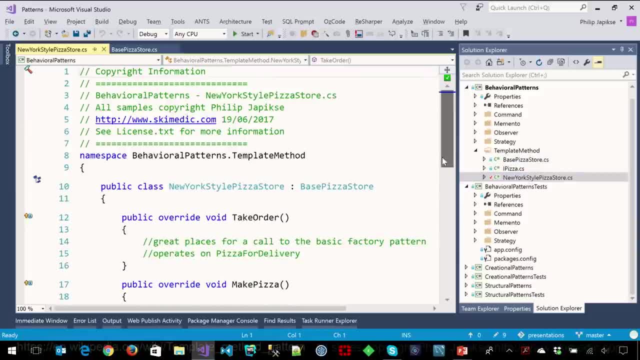 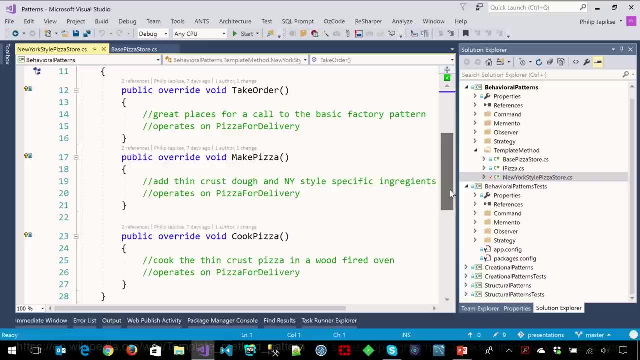 So that really needs to be subclass. So I've got my New York style pizza store And there's no real implementation here, cuz again, I'm just trying to show the pattern, Right, okay, But for take order, I'm gonna operate on this pizza for delivery. 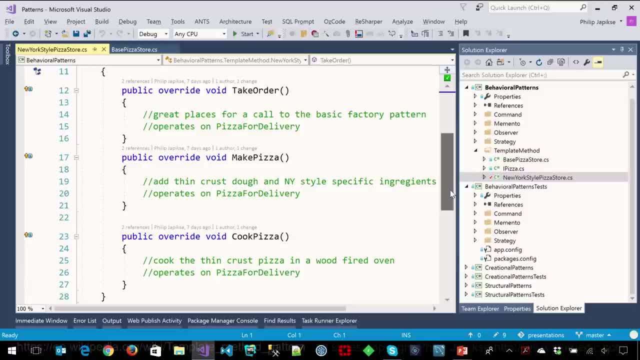 which is defined in that abstract class. That's the IPizza in the abstract class And this is pizza. Okay is probably a great place for the basic factory pattern. We haven't aired that show yet, but it will be coming up as part of this series. 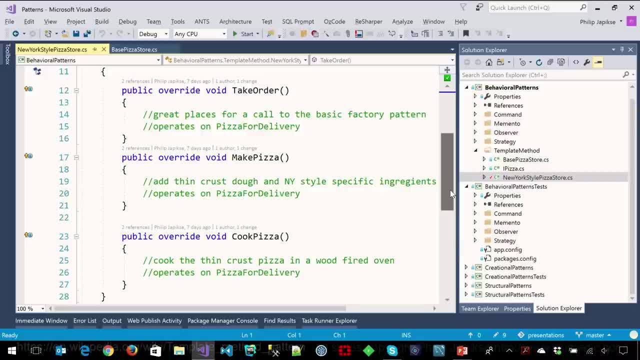 But just know that we're going to return some sort of I pizza, Probably be a thin crust. it's New York style: spicy ingredients, lots of sauce. Then we're going to make the pizza and it's going to be thin crust. 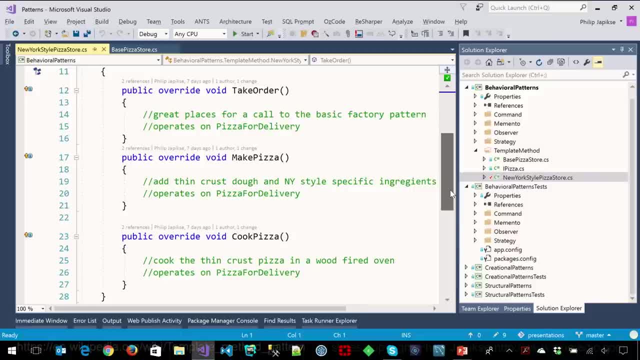 so we have to cook it less. Maybe a Chicago style pizza would have to cook it longer. So it's a specific implementation is deferred to the derived class. So I make and cook. both fall into that, Right Right, So probably cooked in a wood-fired oven for. 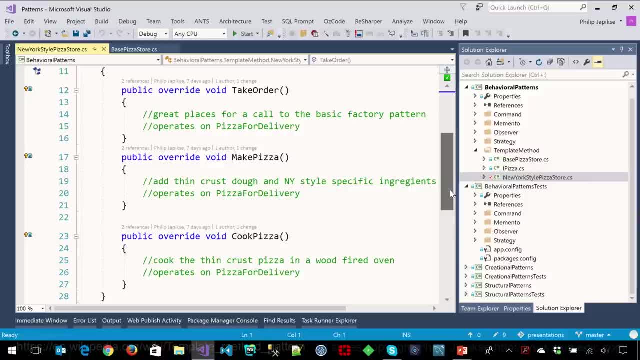 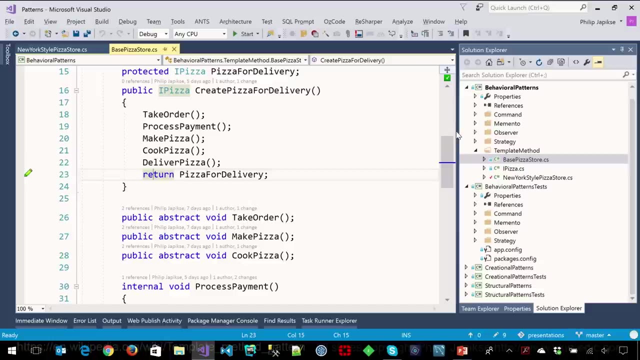 New York style pizza and a different style of onion for Chicago style pizza. Right? So that's the crux of the template method, One thing that you'll notice when we get to the factories. So you would then have a separate class for the various types of pizza. 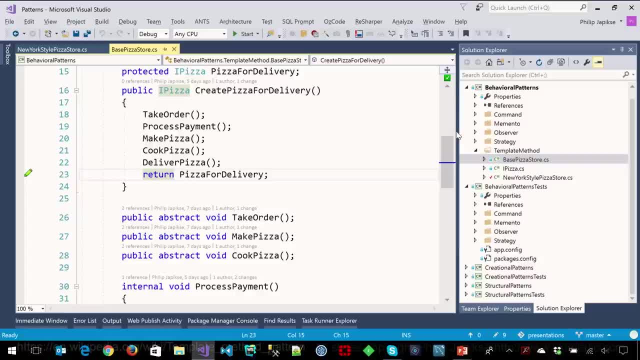 Correct. If you created a new type of pizza that you were offering, you would just have a new implement, a new class, different style pizza store which still has a take order. make pizza, cook pizza: The steps are the same. 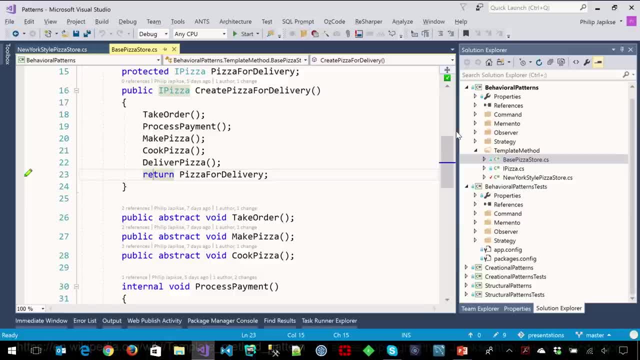 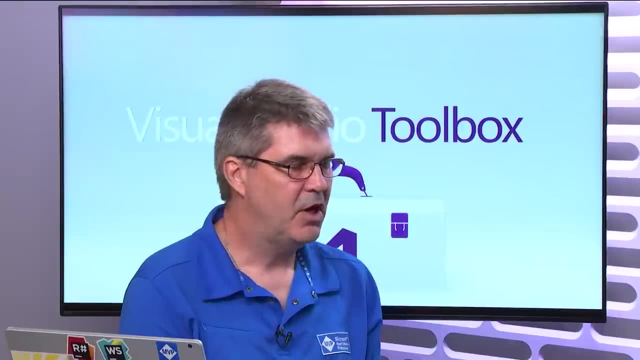 but how you do it is differently, But regardless, you're always processing the payment and delivering in the base class, Correct, Okay, What you just maybe inadvertently called out is one of the problems with the template method is if I have a Upper East Side style pizza. 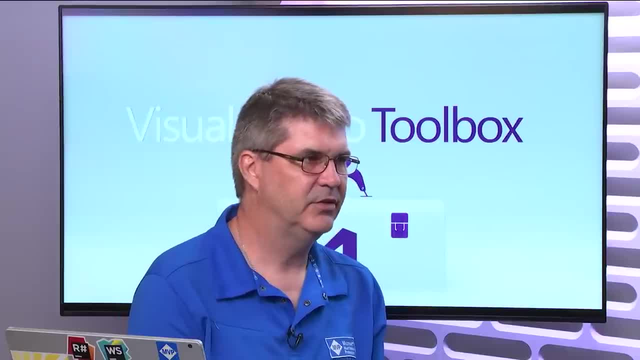 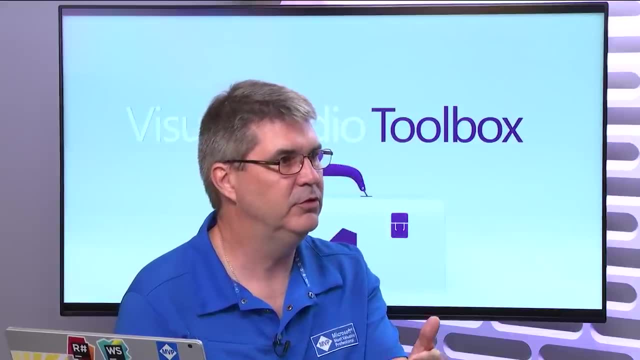 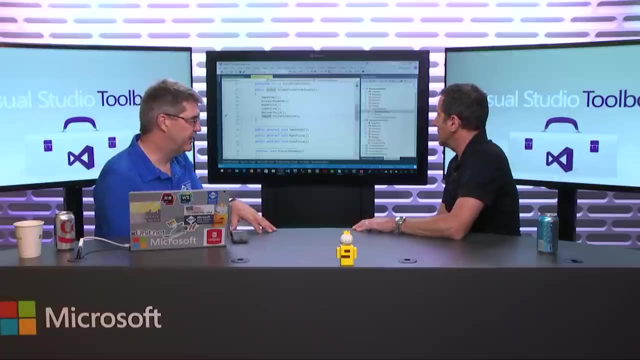 where the only difference is maybe the types of ingredients: not pepperoni cheese, but the type of cheese or the type of pepperoni. now I have to create a whole new derived class to handle that one method. Okay, Right, When we get into the factory patterns. 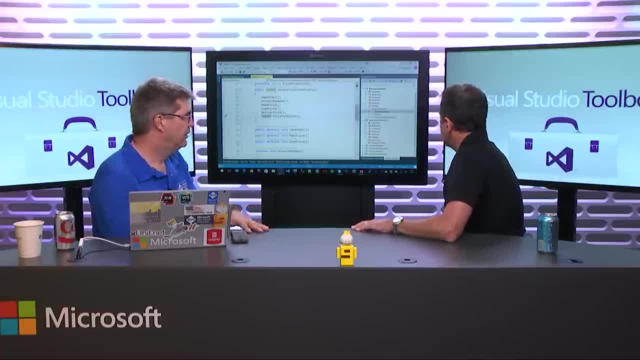 and there's two in an honorable mention, but we'll just call it three. you'll see where it takes a template method and you'll see where it takes a template method and fixes that problem, But for a lot of implementations. this is great because, again, 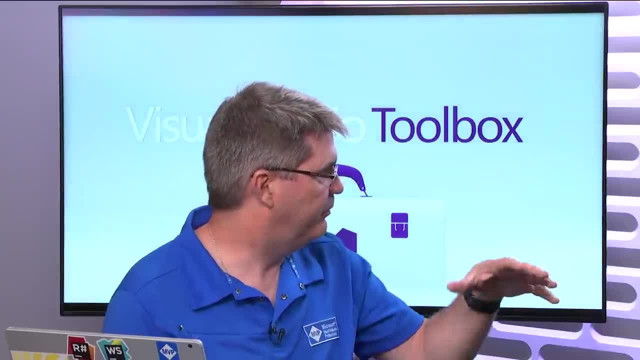 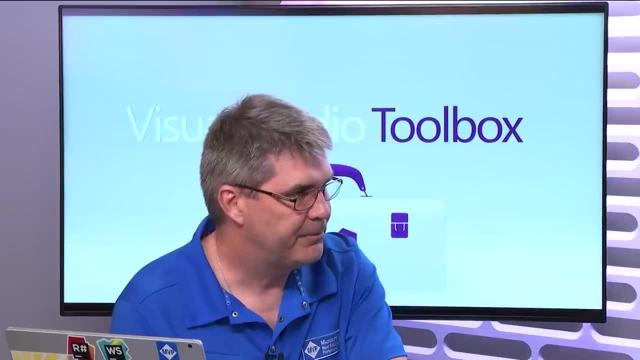 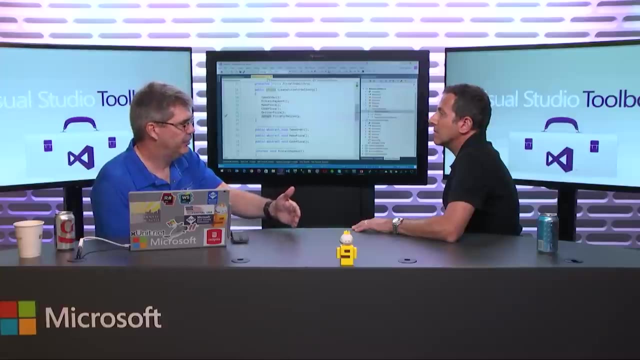 going back to that e-commerce thing, if I have, probably the level I would do, is books perishables fragile, right? So again, taking the order, processing the payment, picking, packing, shipping, But if I know that perishables need to be shipped a certain way. 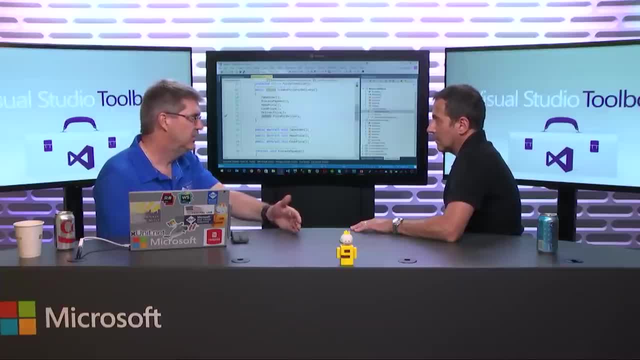 and fragiles versus books or things like that, right. So now we've got the take order and delivery in the base class, So I'm going to send it out to UPS or United States Post Office, or I got to make sure I hit everybody, since you don't have sponsors, FedEx. 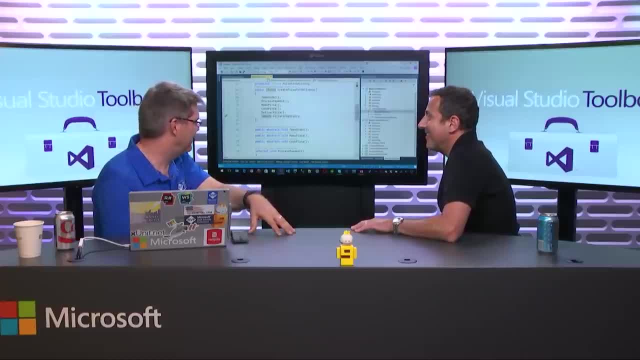 I'll be like NASCAR here. I'll just have stickers all over me for all the delivery companies. Yeah, that would be the template method, right? So we've got this base, But you can have an explosion of classes with this, Right. 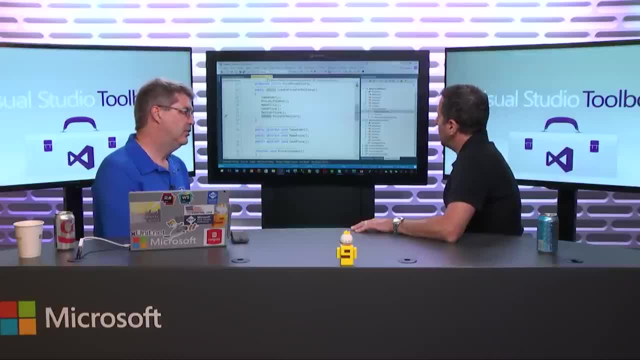 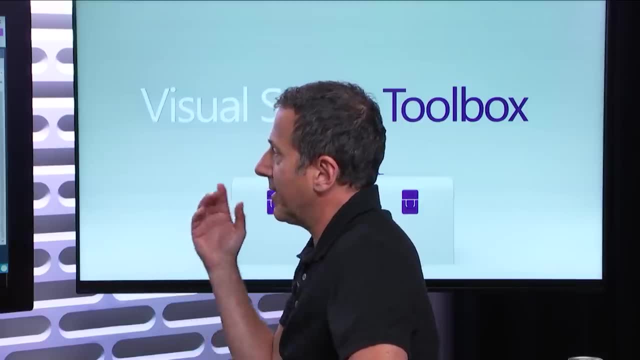 Because every time I need a variation- now I'm making, I'm making another. Yeah, Now I could also implement this using the strategy pattern. right Where I can, I where the take order, make pizza and cook pizza. change at runtime. 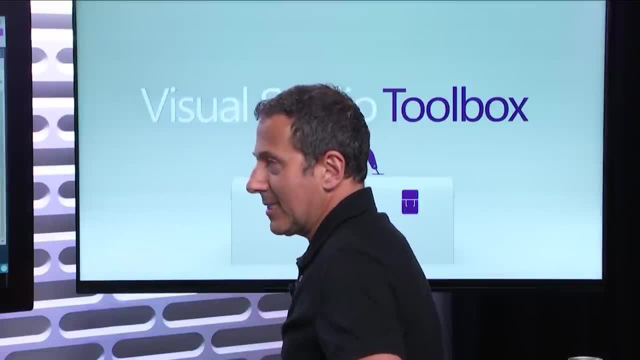 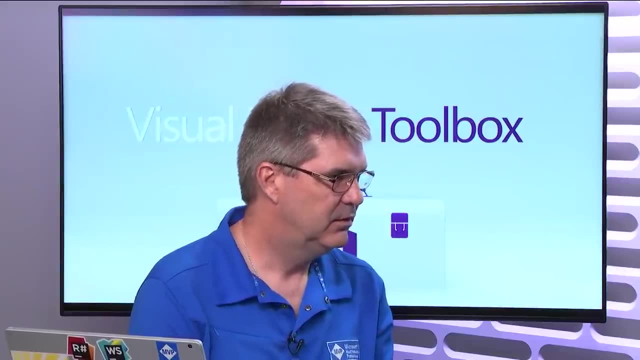 based on the type of pizza that's being ordered. Yes, We covered the strategy pattern in the previous episode, So how would I know which one to use, or how would I decide? Well, some might say it's a coin flip, Okay. 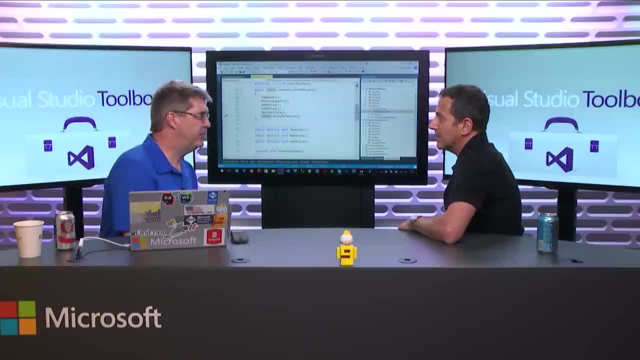 I would say that this is probably not the strategy pattern, because you're really not changing at runtime. You're going to know ahead of time that this type of pizza gets cooked this way. Okay, This other type of pizza gets cooked this other way. 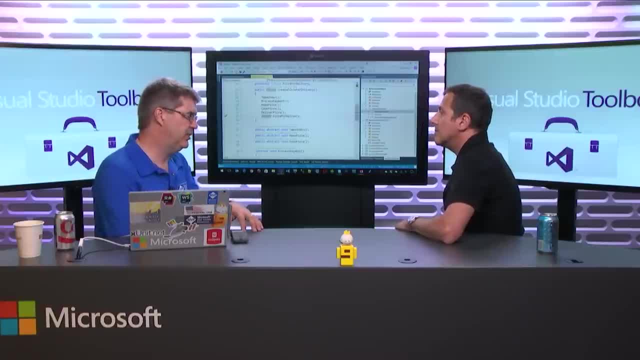 Now, if you wanted to take a Chicago-style pizza and not cook it all the way, then maybe that's a strategy pattern, right? Or maybe you should just make pizza the right way. Well, or you're stuck in a hotel that doesn't have. 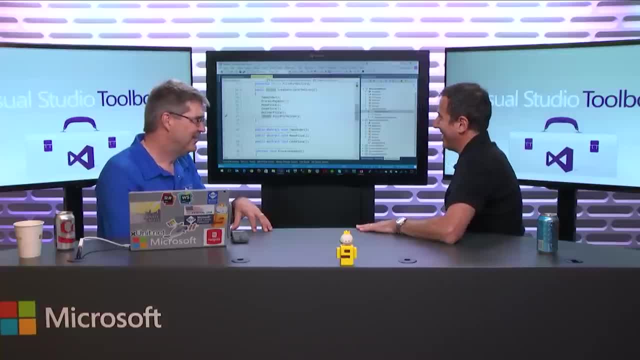 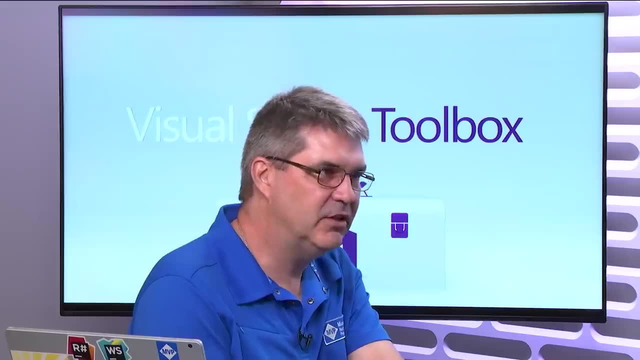 an oven and you bought a DiGiorno pizza and you're trying to cook it in a pan, So which, by the way, doesn't work, I can tell you from experience. So, but that's changing implementation at runtime as opposed to at design time. 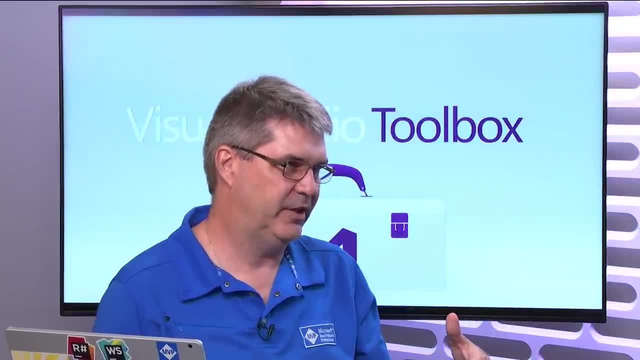 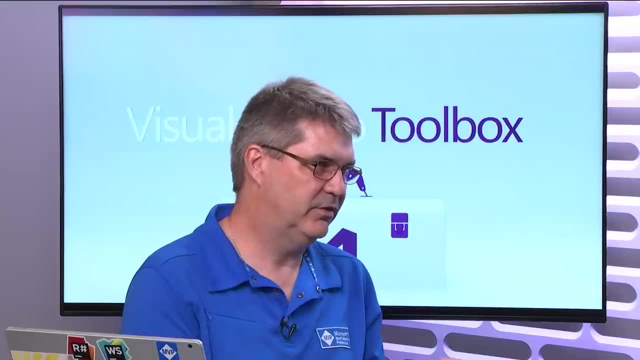 Got it So at design time. I'm changing it because I'm pulling in a different class Right. I'm instantiating a different object of that interface. Got it Right At runtime. it's still for the strategy pattern. 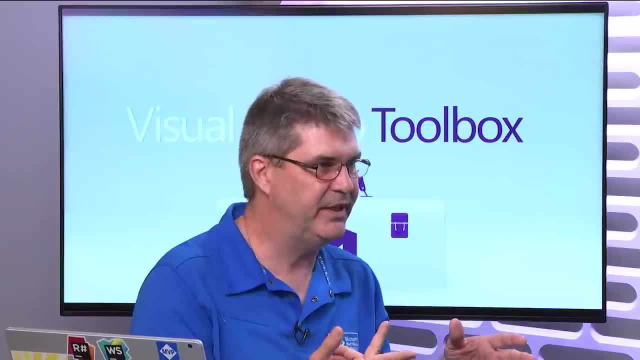 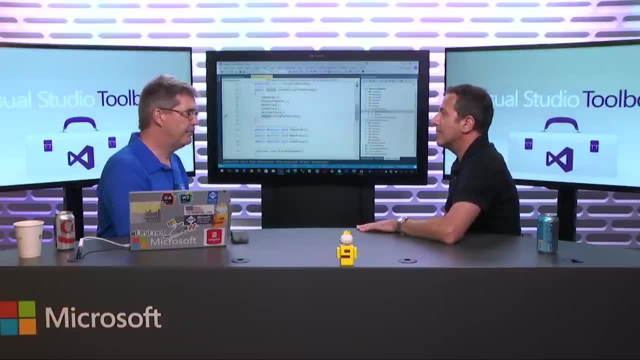 it's still the same instance. I'm changing its behavior at runtime, not picking a different implementation detail. Okay, Makes sense. Yeah, So we talked about some of the drawbacks that you could have code creep right In- just explosion of classes. 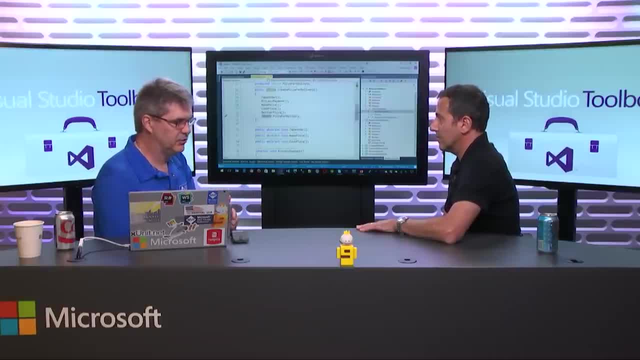 But this is the first time we mentioned patterns aren't in isolation. normally Some kind of are like the simple factory pattern. you don't normally combine with a lot of others. But even when we look at this, what kind of screams out at you where I've got? 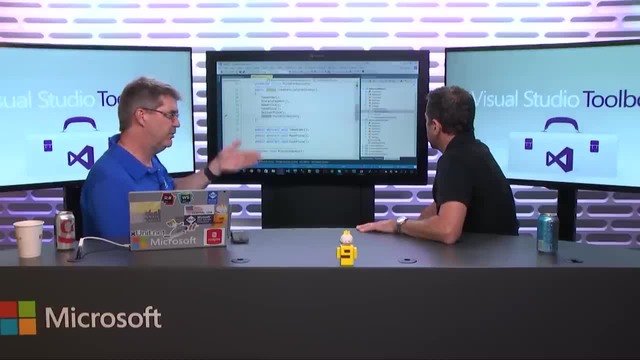 take order and make pizza and deliver pizza. You already said it. That's like the command pattern, right? Yeah, Go do something. I don't care how it gets done Right, Just go do it right. So now we've got the command pattern. 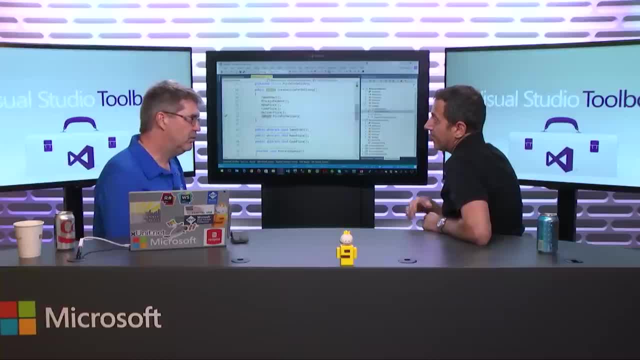 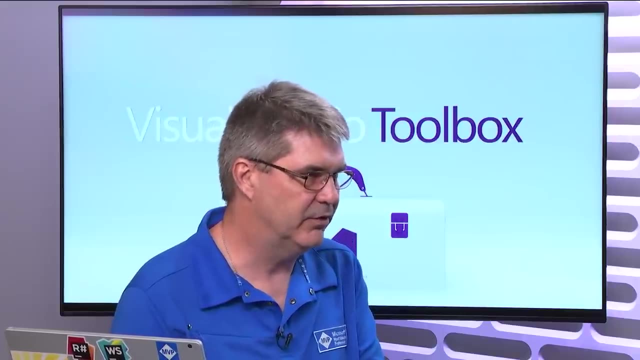 tying into the template method. Yeah, We're also going to see that in the factory patterns and lots of different places. So, while the command pattern and memento were pretty simple to talk about, the reason I felt they needed their own show is because they're foundational to so many others. 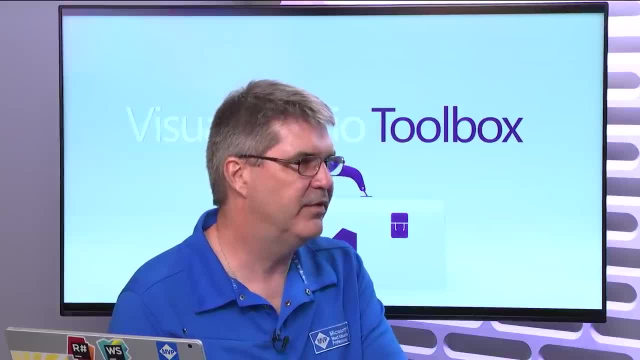 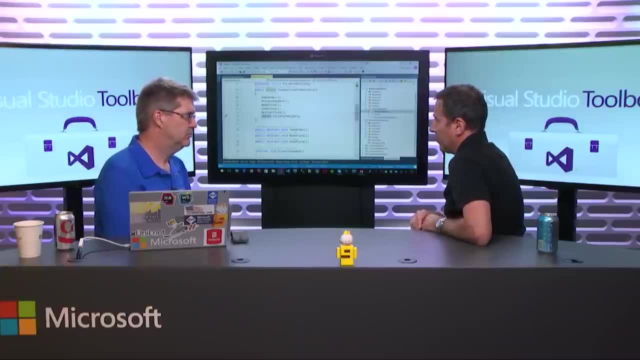 Okay, And we're going to keep seeing this recurring theme of how these all work together. So let's say, process, payment and delivery. pizza also changed based on the type of pizza, So all five of these methods were in a different class.